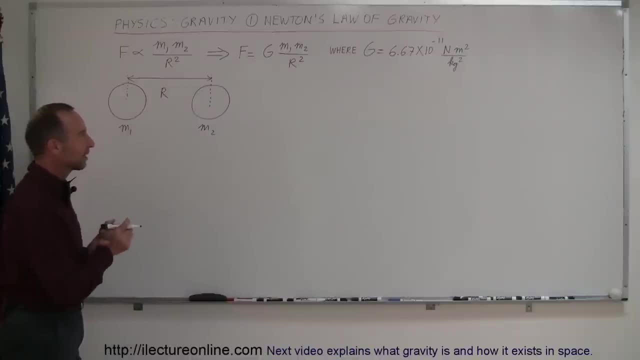 So we're going to talk about gravity, of course in a little bit more systematic and scientific way, starting out with Newton's law of gravity, or Newton's law of universal gravity, as they say. And so Newton at some point discovered that there is a force between any two objects. 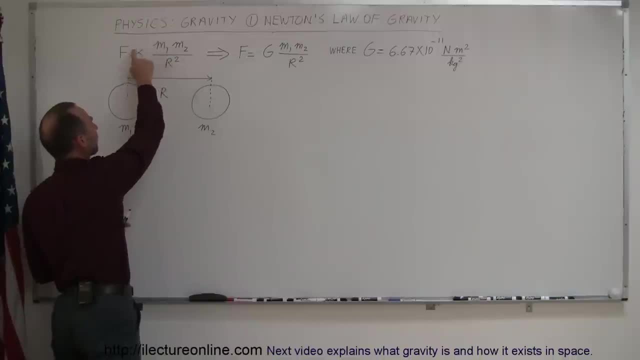 it's proportional to the product of their masses and inversely proportional to the distance between them squared. And when we talk about the distance between two objects, we are talking about the distance from the center mass of the one object to the center mass of the other object. 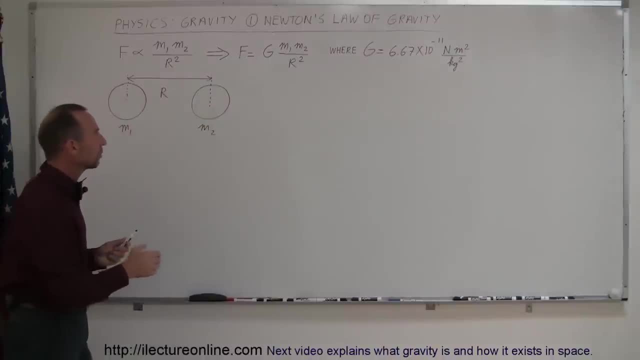 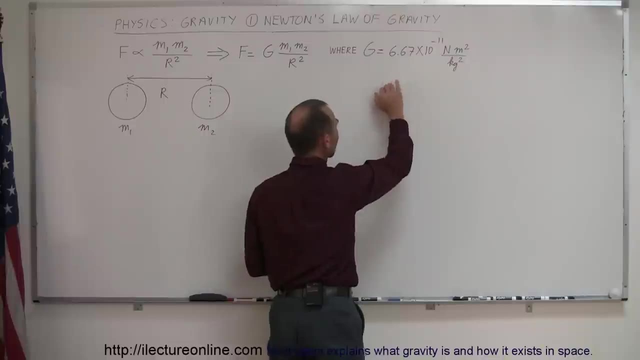 To turn that into an equation, we have to come up with a constant and of course g is now considered to be the universal constant of gravity. g is now measured to three significant figures, to be 6.67 times 10, to the minus 11 newtons times meters squared. 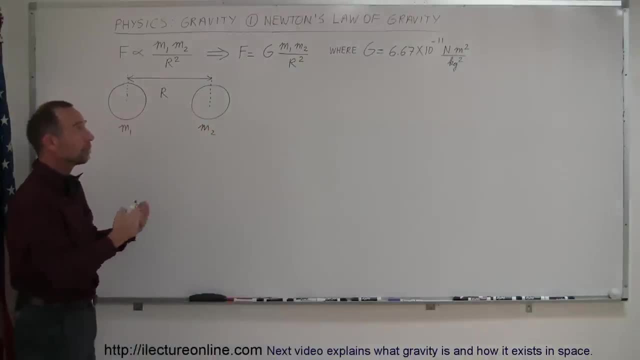 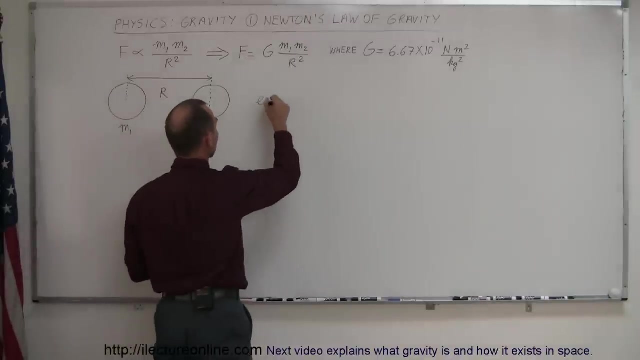 per kilogram squared. Now how do we apply that? Well, we apply that by saying: if we have two masses of some of some known quantity, separated by some known distance, we should be able to figure out the force between those two objects. So as an example, let's try that example. Let's say that 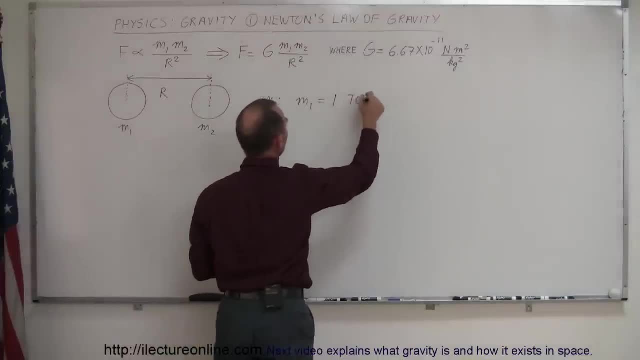 mass one has a mass of one ton which, by the way, is 1,000 kilograms. Let's say that mass two also has a mass of one ton which, by the way, is 1,000 kilograms. Let's say that mass two also has a mass of one ton which, by the way, is 1,000 kilograms. 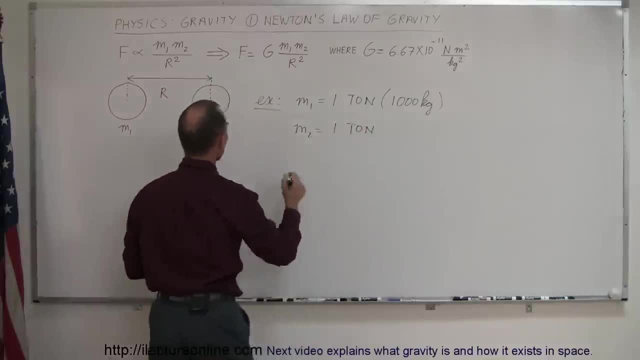 has a mass of one ton which, by the way, is 1,000 kilograms. Let's say that mass two also has a mass of one ton, which, by the way, is 1,000 kilograms. So we know it's 1,000 kilograms. and let's say that the distance between them equals 5 meters. 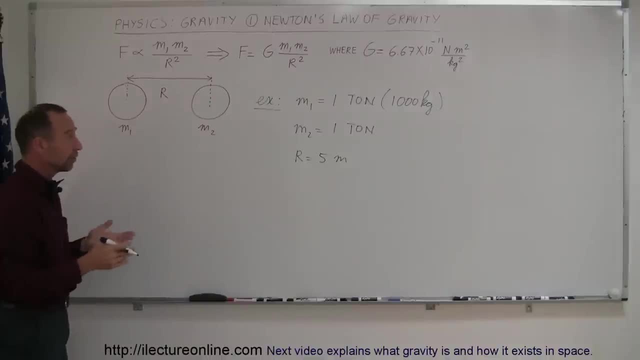 So what would be the force between two such objects? Now, a ton is almost the weight of a car- a small car anyway- and five meters apart. So let's say we have two cars five meters apart. What would be the force of attraction between them because of the law of gravity? Well, let's try that. 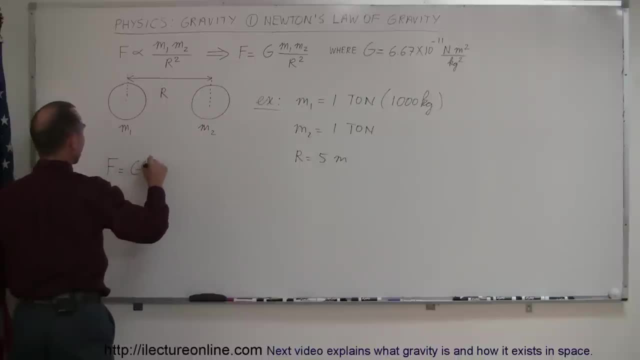 We plug in the equation. F is equal to g times m1, m2 divided by the distance between them. So g is 6.67 times 10 to the minus 11 newtons meters squared per kilogram squared. So g is 6.67 times 10 to the minus 11 newtons meters squared per kilogram squared. 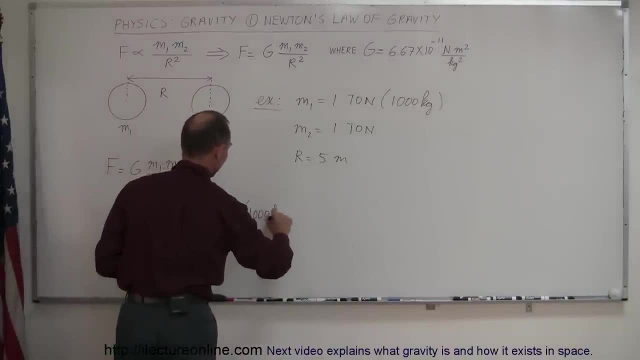 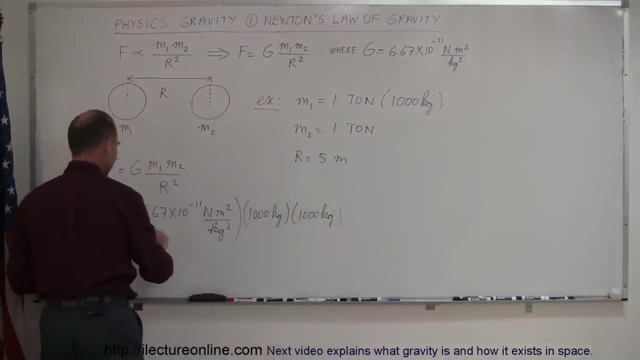 We multiply that times the mass of one, which is 1,000 kilograms, times the mass of the other, which is 1,000 kilograms, times the distance of five meters, which is roughly 15 feet. All right, so we have five meters and we have to square that. 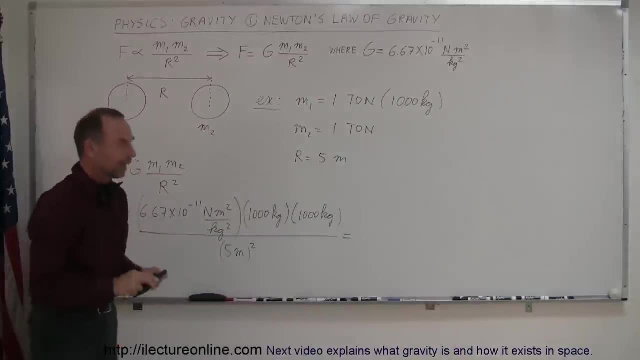 And now, what will that equal? And that's the equation. Yes, you'll find out when we crank out those numbers in the calculator that the result is actually a very, very tiny number. The force of gravity on small objects is extremely minute. 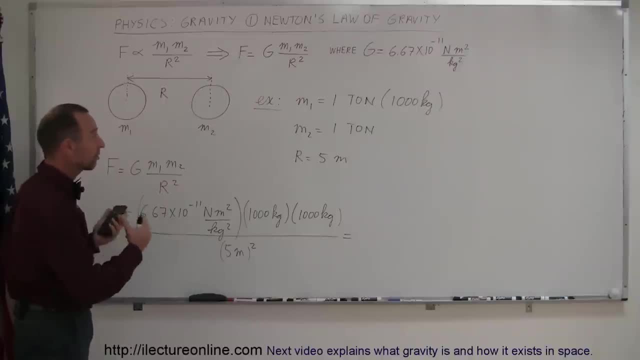 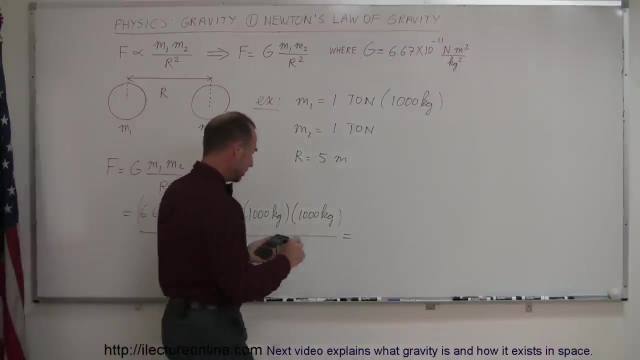 It only begins to exhibit itself on very large objects such as planets and moons and stars and so forth. All right, so we have a 6.67 e to the 11 minus times 1,000.. We can square that: divided by 5, squared equals and yes indeed. 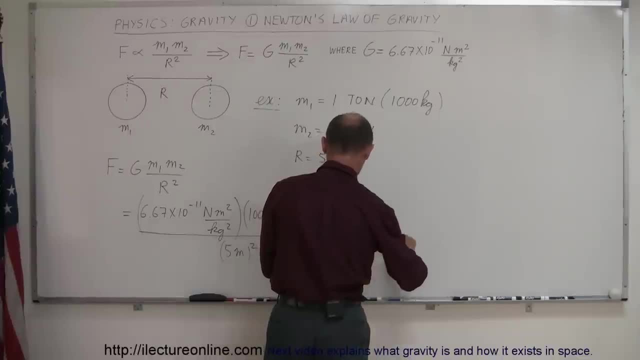 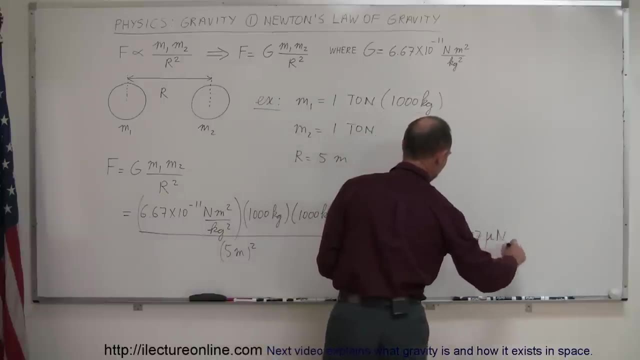 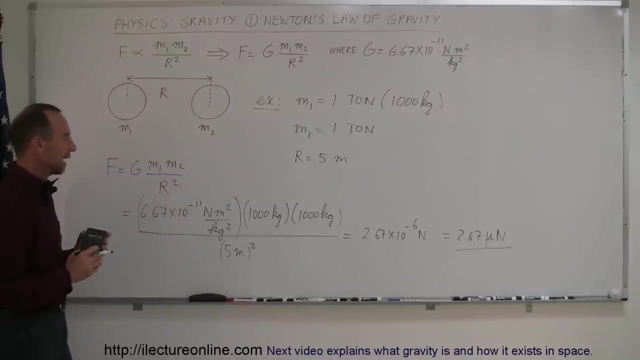 the number is 2.67 times 10 to the minus 6 newtons, which is the same as saying 2.67 micronewtons. Now, that's extremely small force, so no danger of two cars colliding with each other due to the force of gravity. 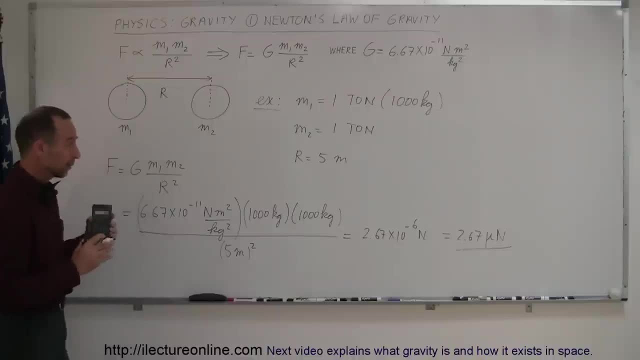 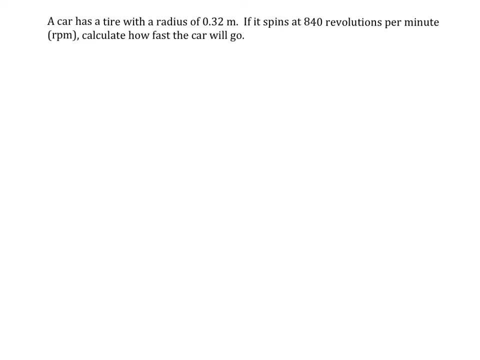 All right, in this problem we're trying to find the speed that a car will travel, and we know its tire has a radius of 0.32 meters and that this tire is going to spin at 840 revolutions per minute, And so we want to find out how fast the car is going to go. 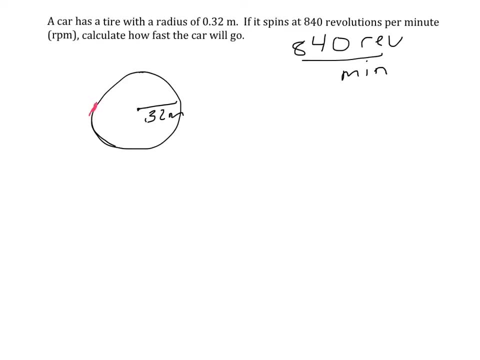 So this is really asking how fast, if you had something stuck on one of the tires, how fast this is going around in the circle, Because that's on the road that essentially is going to be. however fast this is going here, that's how fast it's going to move on the road.